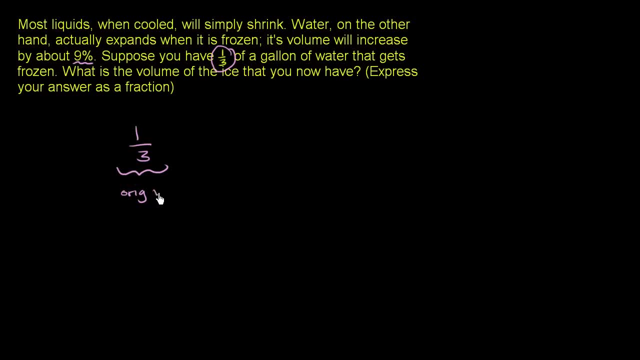 So this is the original volume- 1 third of a gallon- And it's going to expand by 9%. So your frozen volume is going to be your original volume plus 9% of your original volume. So plus 9% of your original volume. 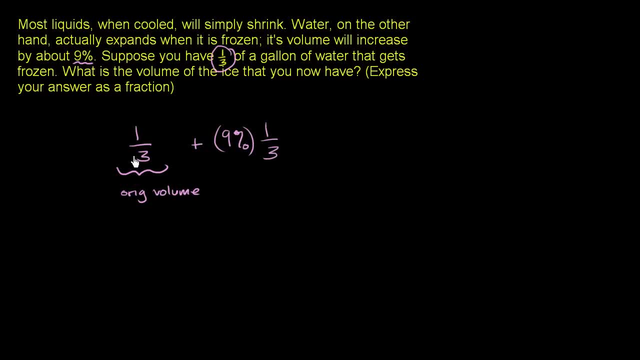 So you could say it's 9% times 1 third. So this right over here is going to be the expanded volume. Now there's a bunch of ways we can figure it out. We could turn things to decimals or whatever else. 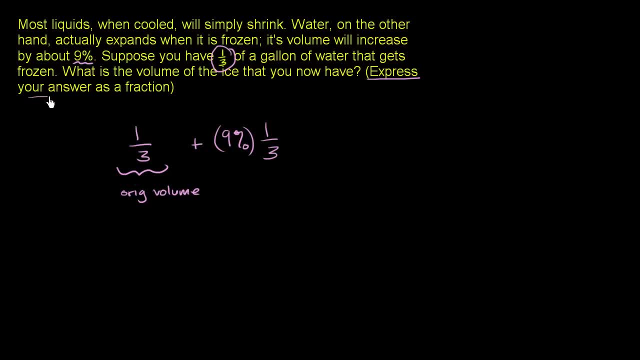 But they tell us to express your answer as a fraction. So let's make sure that everything here is a fraction, And then we'll just try to simplify. So the one thing that's sitting here that is not a fraction is our 9%. 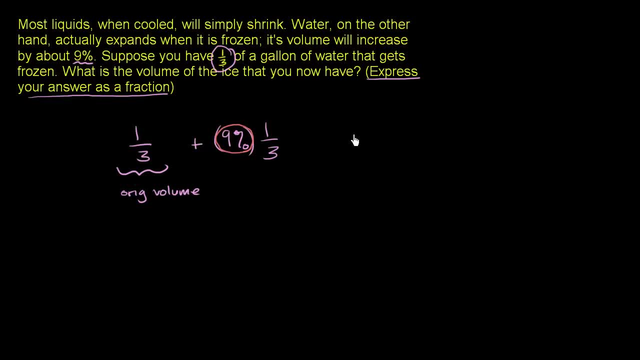 Well, what does 9% actually represent? Well, 9% literally means 9 per 100.. So we can rewrite this. So this is going to be equal to 1 third plus, instead of writing 9%, I'll write that as 9 per 100.. 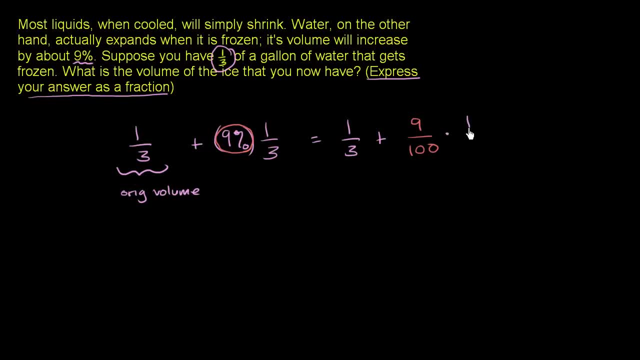 And then once again times 1. third, And we can simplify this expression right over here- We have a 9 in the numerator, a 3 in the denominator. If we divide both of them by 3, we get a 3 and a 1.. 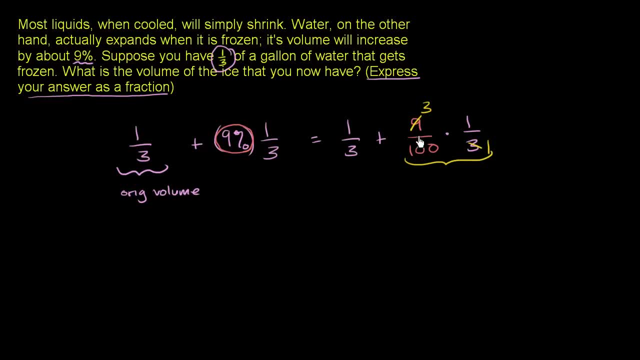 And so we're left with 1 third plus 3 hundredths times 1 over 1.. Well, that's just going to be 3 hundredths, So this is just going to be equal to 1 over 3 plus. I'll write this in orange still, or maybe I'll do it. 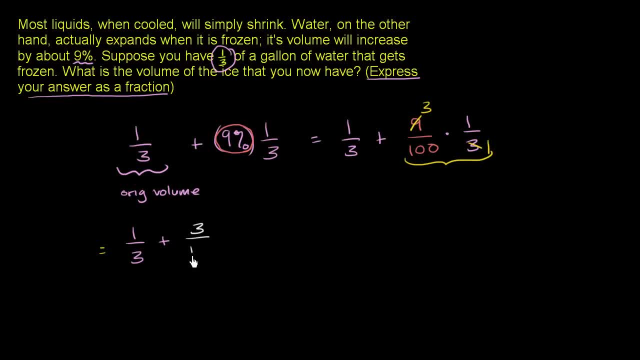 in a new color, plus 3 over 100.. And now we have to add two numbers that have different denominators. So let's find a common denominator. So this is going to be equal to well, the least common multiple of 3 and 100. 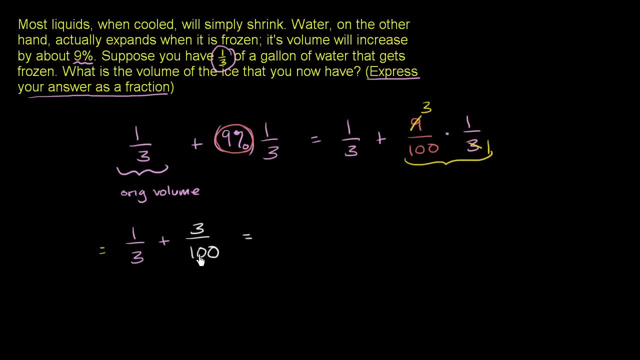 And they share no common factor. so it's really just going to be the product of 3 and 100.. The least common multiple is 300. So it's going to be something over 300 plus something over 300.. Now to go from 3 to 300 in the denominator. 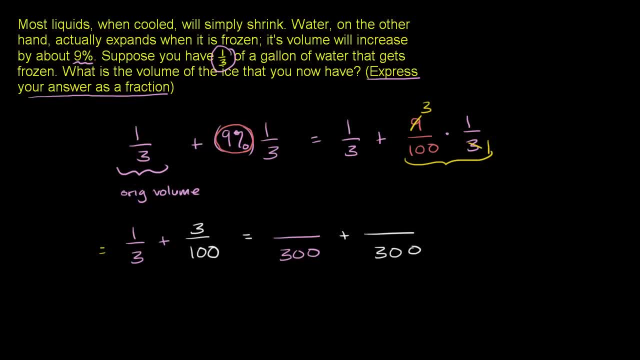 you multiply by 100. So you have to multiply the numerator by 100 as well. So 1 third is the same thing as 100 over 300. And to go from 100 to 300, we had to multiply by 3 in the denominator.